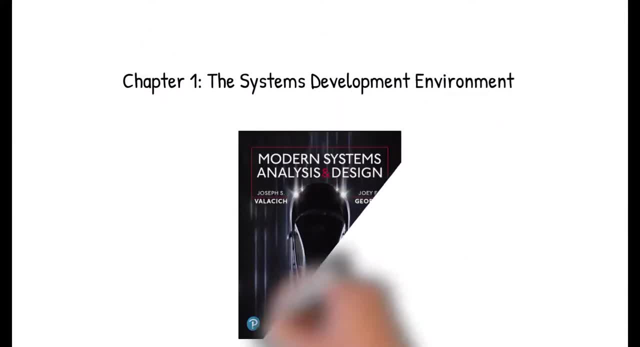 Chapter 1 gives us an overview of the systems development process. You probably haven't thought much about how systems or software applications are put together or developed. You're probably aware that there's some coding involved, as well as some internal or alpha testing, and there may be some beta testing as well, but that's just part of the whole picture. 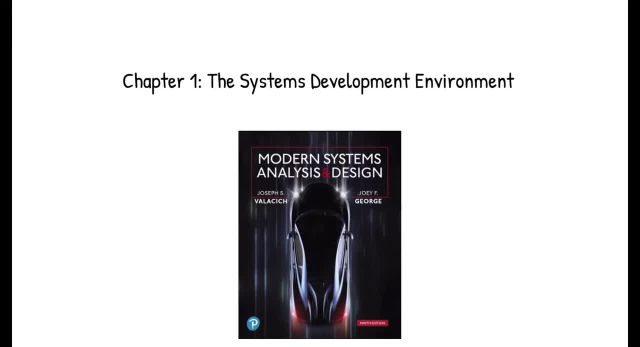 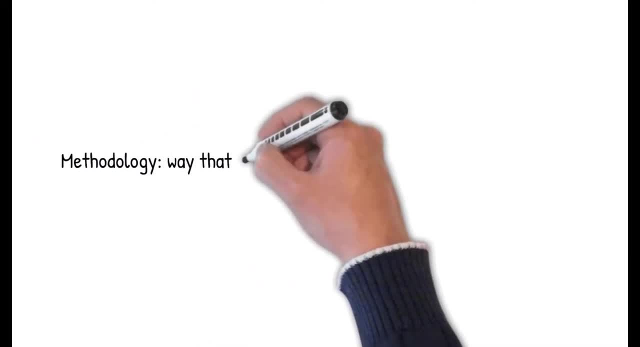 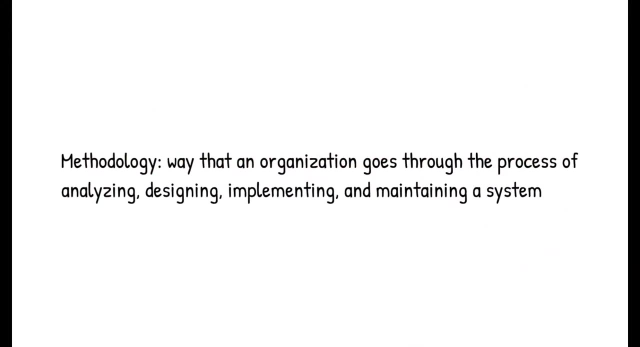 behind systems development. There is a lot of planning involved before any code is written or any networking equipment is purchased. When we talk about methodologies, we're talking about ways that an organization goes through this process of analyzing, designing, implementing and maintaining a system. There are several methodologies out there today, and each one 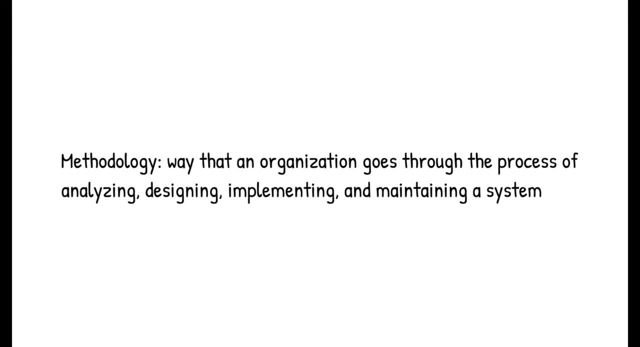 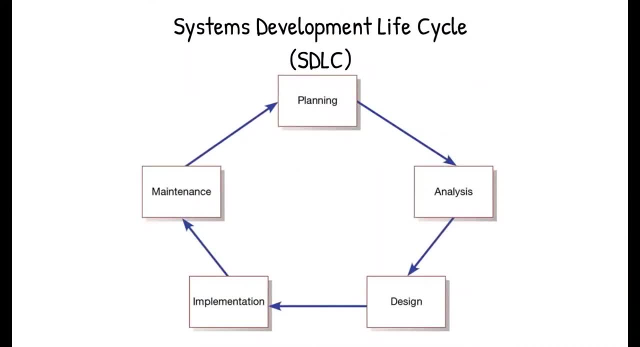 has its usefulness depending on the situation. The oldest model is the Systems Development Lifecycle, or SDLC. This is distinguished by its distinct and discrete phases consisting of planning, analysis, design, implementation and maintenance phases. It's cyclical in nature, in that the end of the useful life of one system leads to the start of the next. 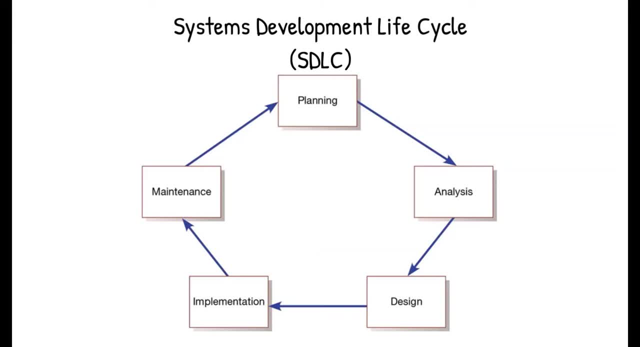 If we were to look at Windows, for example, we can see how this works out. Windows 8 went through a process like this, as it was being prepared for the public, and once it hit the shelves, the development team fixed bugs and released service packs. 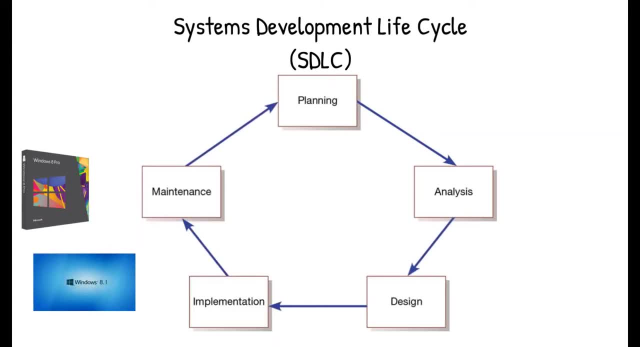 and eventually Windows 8.1,, which was a very long process- was a very long process. At some point, a decision was made to come up with something completely new because there were too many bugs to fix or because there were new technological developments. 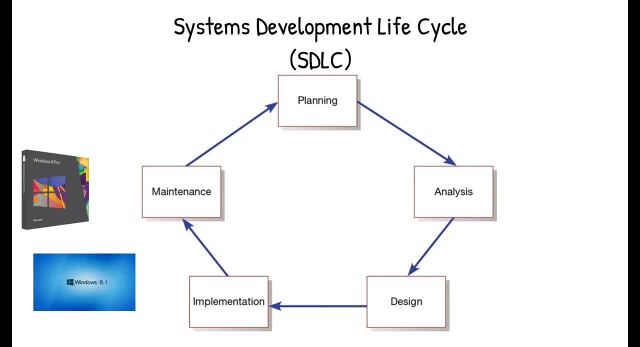 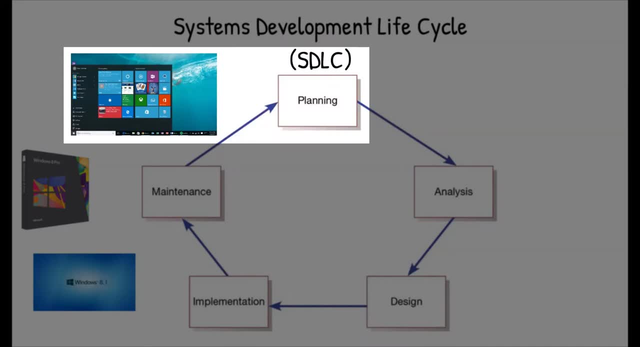 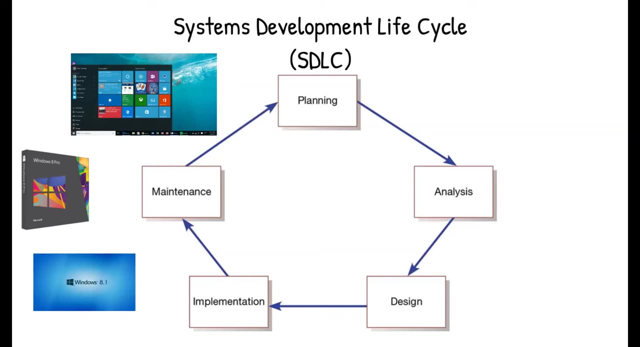 or whatever the reason may be, moving us from the maintenance phase back to the planning phase to start a new product, which eventually became Windows 10.. The SDLC isn't always a five-phase process. Some organizations might combine phases and others might add one or two, depending on their needs. The names of the phases might not even be the same. 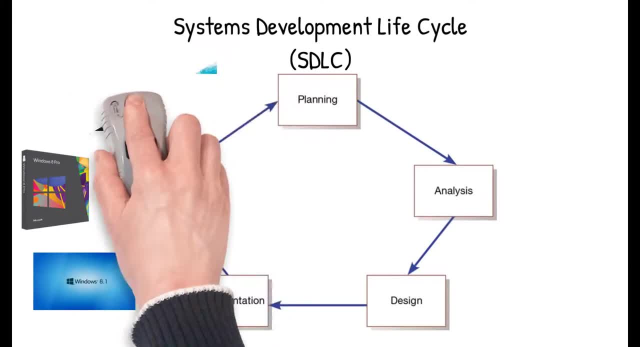 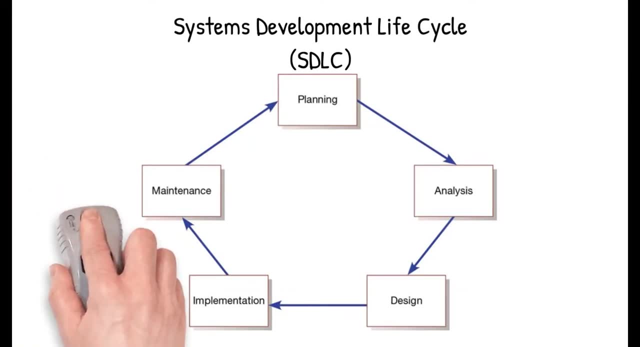 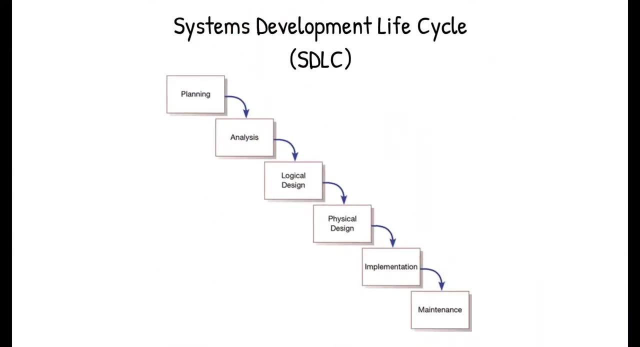 from organization to organization, but the ideas behind them are the same. If you understand the general flow behind projects that follow the SDLC, you'll be fine. In some places you might find the SDLC referred to as the waterfall model. Some organizations think of the process in a linear fashion rather than a circular one. 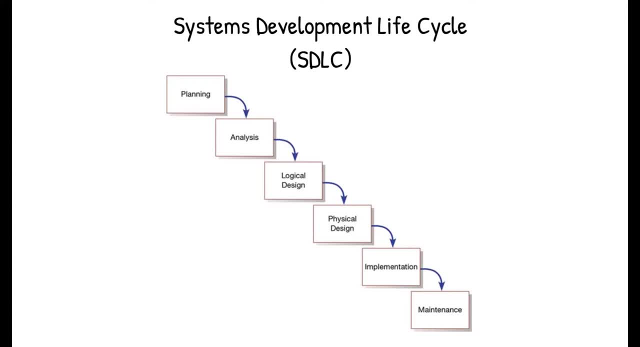 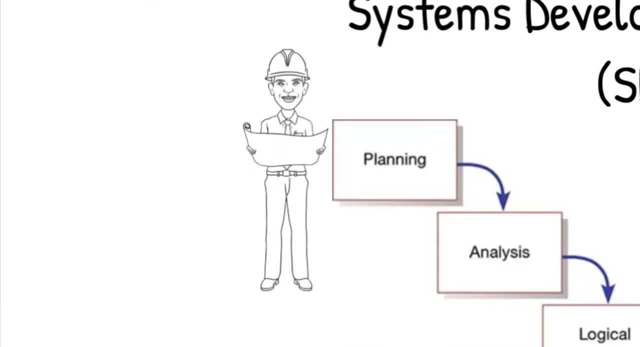 The concepts behind the different phases are different, but they're not always the same. The are the same in either case. The planning phase involves figuring out what projects are important to an organization, discussing the problems to be solved and developing a rough idea of what the 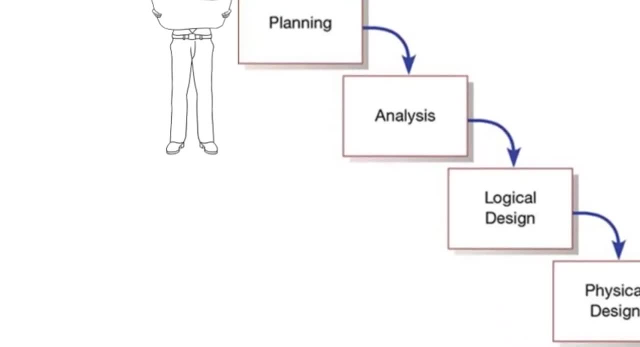 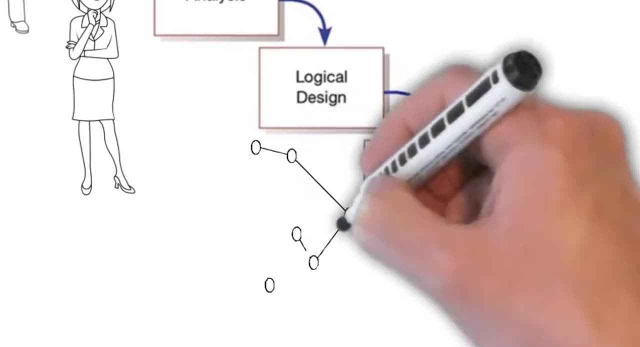 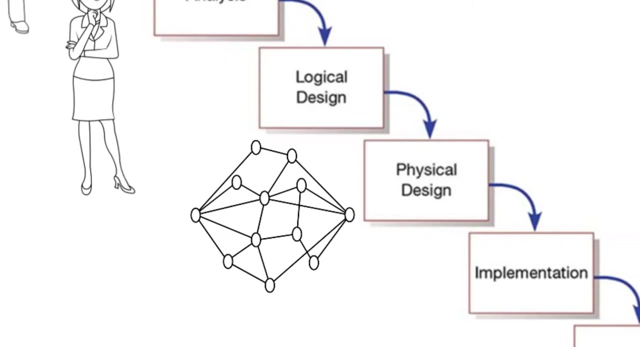 end result will be able to do. The analysis phase dives deeper into the problem and starts to detail what the requirements will be. The design phase lays out what will be needed to make this happen in terms of the specifications of the hardware and software, and where everything can be procured. 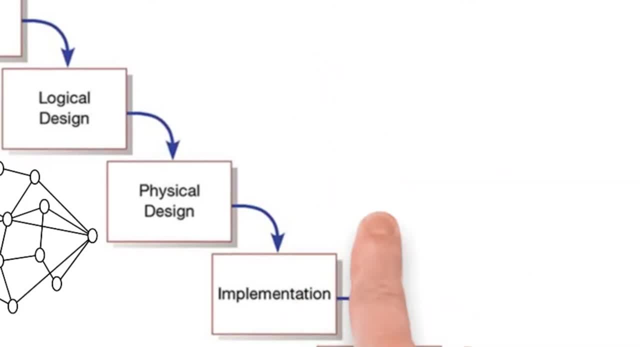 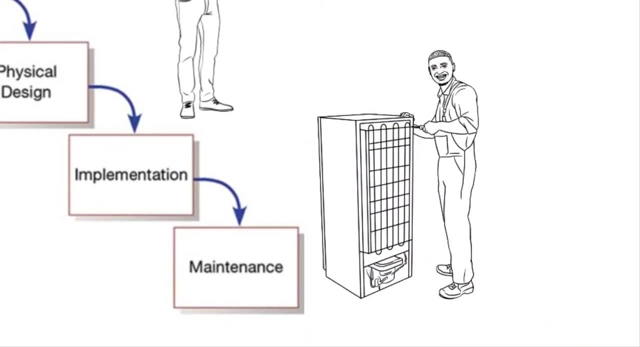 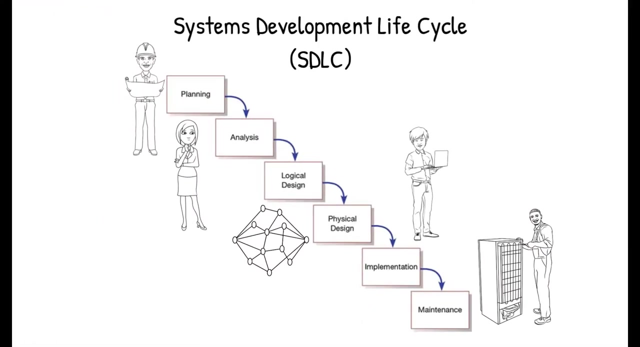 The implementation phase is where all the work gets done and the maintenance phase is where any problems or bugs are fixed. We'll get more specific with what each phase does in future chapters, but for now, get a grasp on the general ideas behind each of the phases: The methodology, 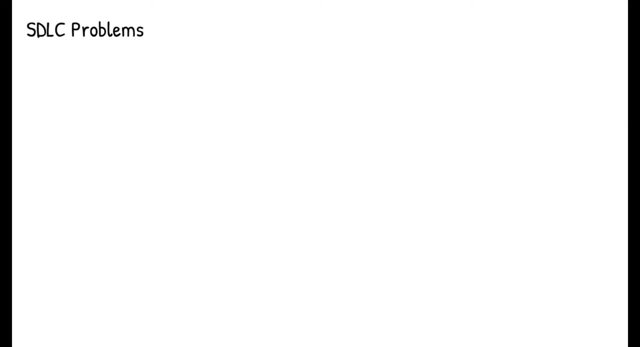 can get problematic if you follow it the way it was designed. This model was developed back in the early 1960s as a means of controlling government projects, And the intention was to make sure that at each phase there were clear objectives or milestones to meet and a way to get out of the project if things weren't going as planned. This rigidity can 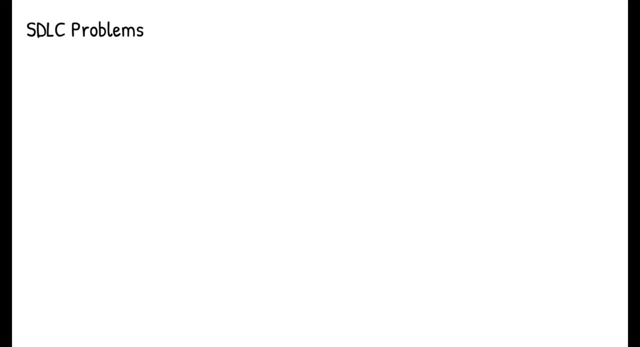 lead to issues. For example, if you're on the design phase, you should already know what the design requirements are, so that you can start coming up with a plan to meet those requirements. You should know that your system will need to be accessible on mobile devices. 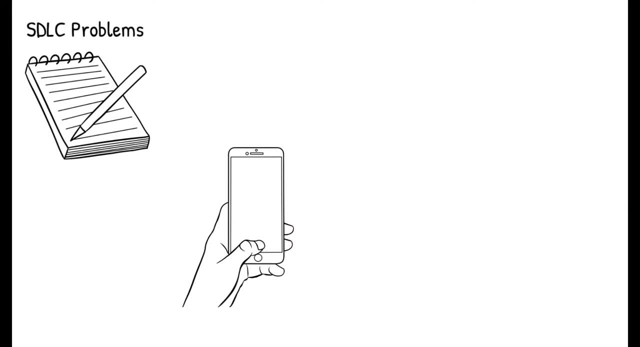 and take both biometric authentication as well as your typical username and password combinations. These requirements originate in the planning phase, but are typically fleshed out in the analysis phase. If someone wanted to make changes to those requirements, that could possibly have a huge impact on the design aspects. So, generally speaking, 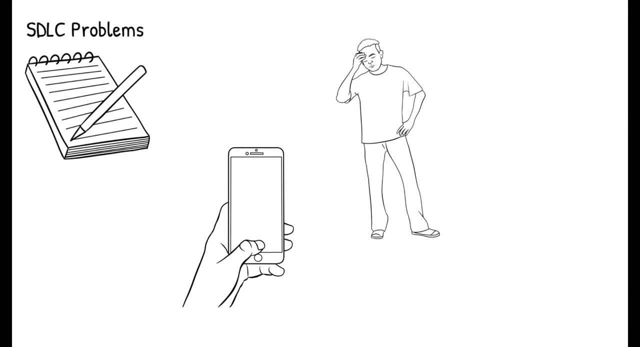 changes need to go through a vetting process before they're accepted. as part of the requirements, There's also a heavy emphasis on meeting deadlines. We'll see in future chapters that changes to the timeline will affect the budget and the scope of the project, which in turn, could affect the overall 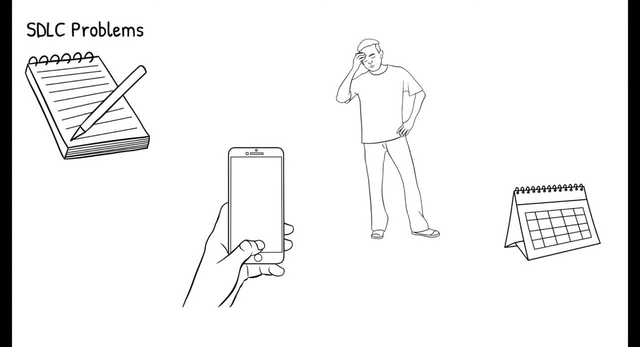 quality of the project. All this doesn't make the STLC obsolete. This methodology can be useful if you have large projects with many different sub-development efforts, or it can be useful if you have a specific idea of what the end result is supposed to do or look like. 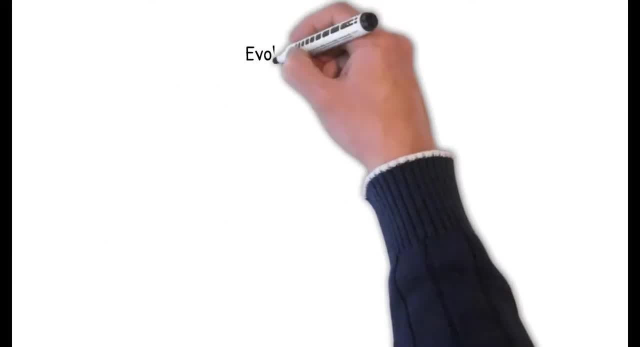 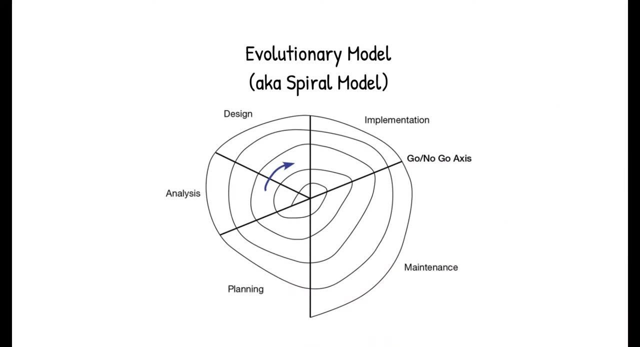 For smaller projects, there are other options. Evolutionary models are sometimes known as spiral models because of the constant change in the design process. For example, if you're on the design phase, you'll see a constant iteration involved. Evolutionary models sometimes use the same. 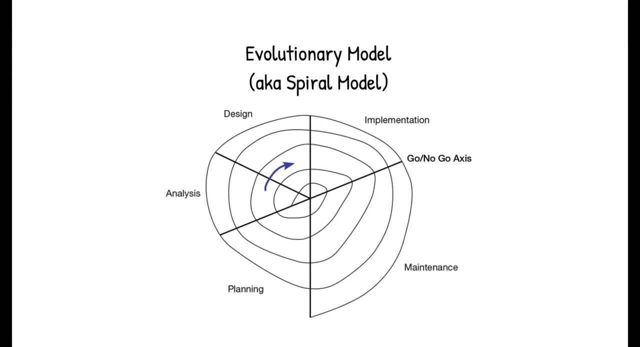 phases in the STLC, but the key difference is that there isn't really a specific end goal to meet by the time you get to the maintenance phase. At that point you can decide to add or remove features based on user feedback. Many games are developed using this concept. A company may put out a beta. 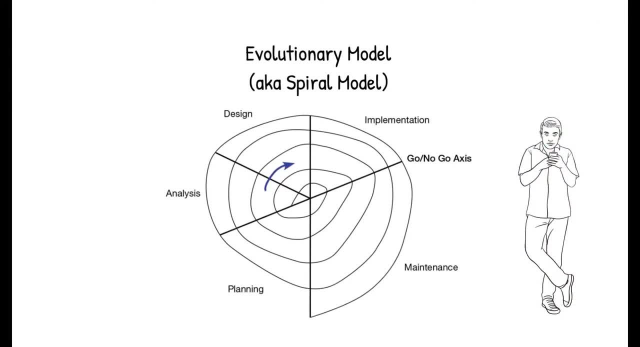 version, get feedback, re-release, get more feedback and then go wide release. This model gives the team a lot of flexibility in terms of getting just the right features in place while creating different prototypes to analyze their work. But the more cycles you have, the longer a. 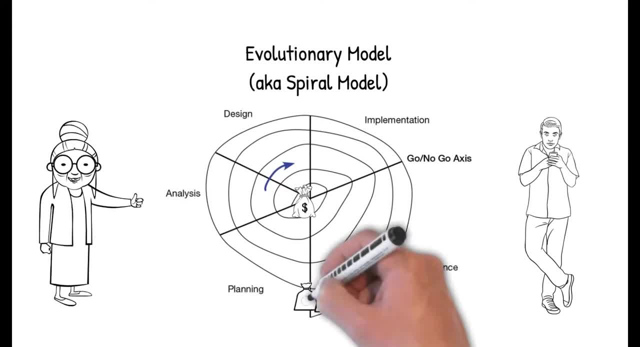 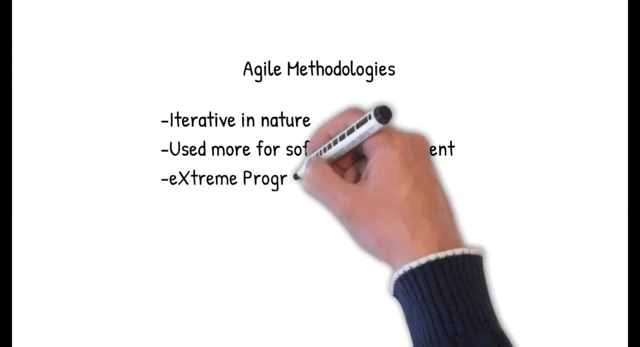 project goes and the more you spend on that project. Agile methodologies also follow iterative methodologies, and these models aim to have a project completed as quickly as possible. Like the spiral model, agile methodologies can be used for projects where requirements are unpredictable And you need to have heavy involvement from your development team, as well as the end users or 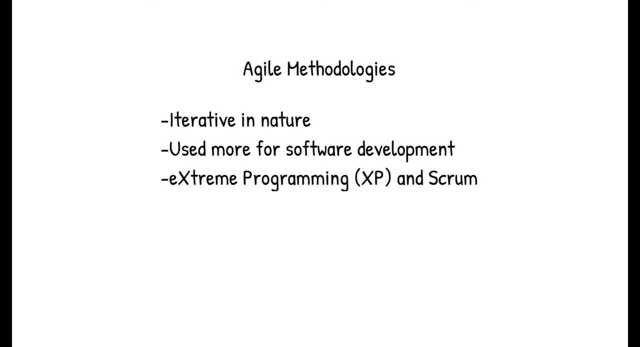 customers. Agile methods are more for software development versus systems development, which may include new hardware infrastructure in addition to software applications. Two of the more popular agile methodologies are extreme programming and scrum. Two other methodologies are object-oriented analysis and design, and relational unified. 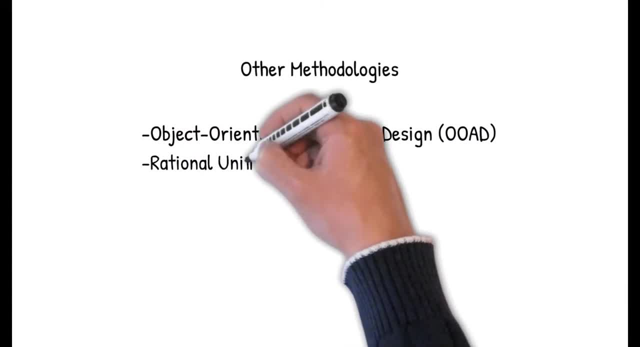 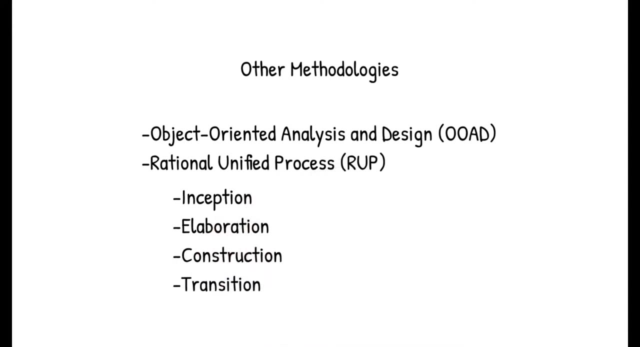 process. Both share commonalities with object-oriented programming, where you deal with objects, methods and inheritance. RUP follows a four-phase model: inception, elaboration, construction and transition- which, when you break down what happens in each phase, 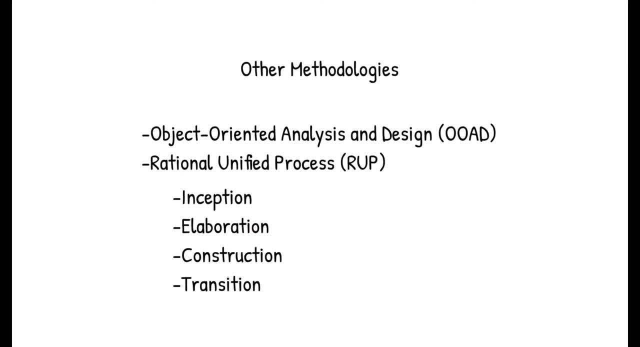 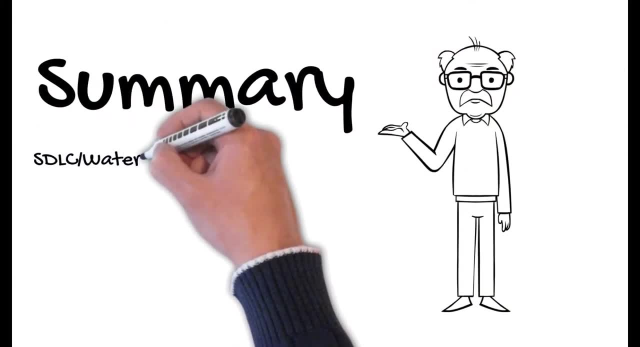 has a lot of the same characteristics as the SCLC. In summary, be familiar with what a development methodology is and the general steps that the SCLC follows. Also know that there are different models that organizations use, including SPIRAL XP.